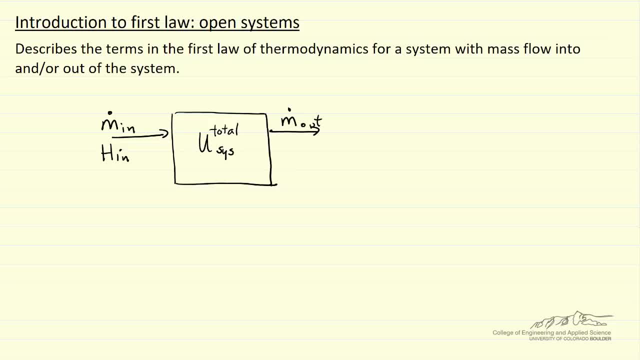 And then we have a mass flow rate out, but it does not have to be the same as the mass flow rate in, because we're looking at general situation and the enthalpy in general is going to be different, The composition can be different, 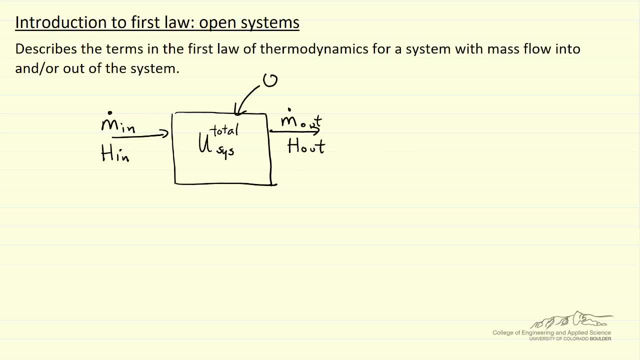 Lots of things can be happening in a system. One of the things is we're going to be adding heat in general, and so the dot would mean this is joules or kilojoules per second, so it's per time We could be adding shaft work. 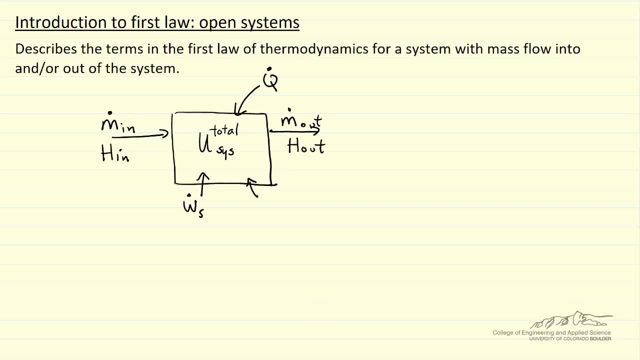 For example, if we have a compressor, and again per time we could add expansion compression work, Let's put a dot over it. We're going to add expansion compression work like a piston moving up and down on the system. So if I want to look at the general energy balance, what I'm going to say is that change. 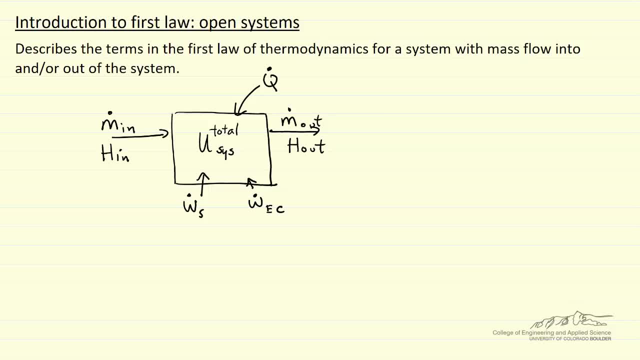 in the energy is a function of how much energy we add, how much energy we take away And what we're going to do here. because we're interested in applications in typical engineering situations, we're going to ignore kinetic energy, potential energy. 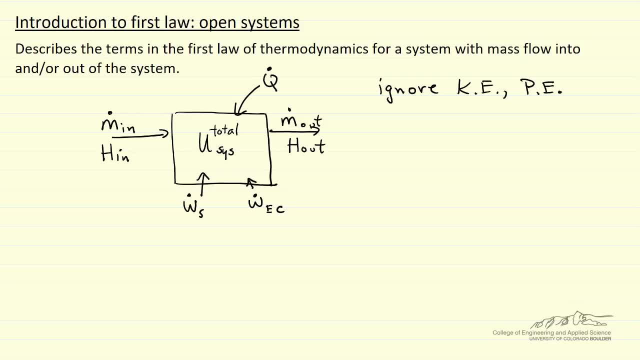 I'm not saying that these terms might not be important in some cases, but the things we're interested in. we're going to ignore these, So we're setting these terms to zero. We could certainly include them if necessary. So then the energy balance says there'll be a differential equation says the change. 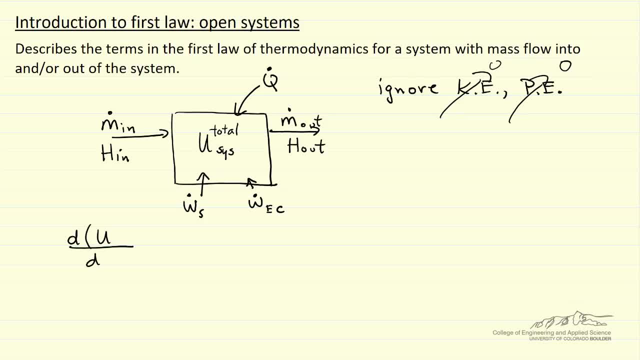 in the internal energy of the system with respect to time, because the temperature can be changing, the composition can be changing. that's due to the fact we're adding energy. So one way we're adding energy is we have low energy And notice this is in enthalpy for the flow term and it's not internal energy. 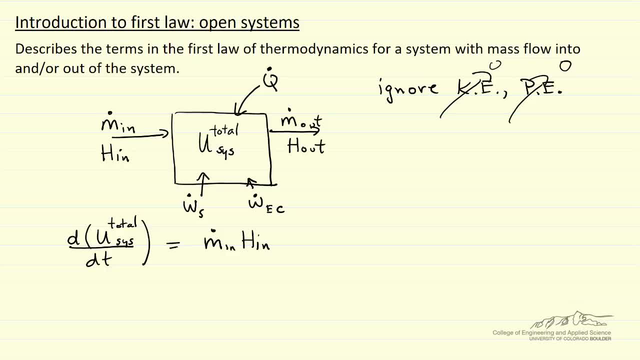 The reason is because of the PV work term. we explained that in other screencasts. So that's one way we're adding energy. One way we're removing energy is we have mass flow out and again that's an enthalpy term. 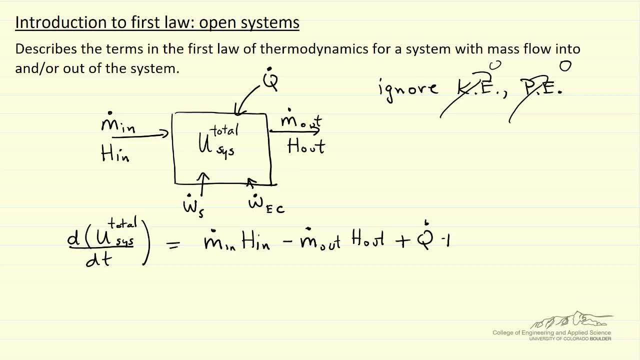 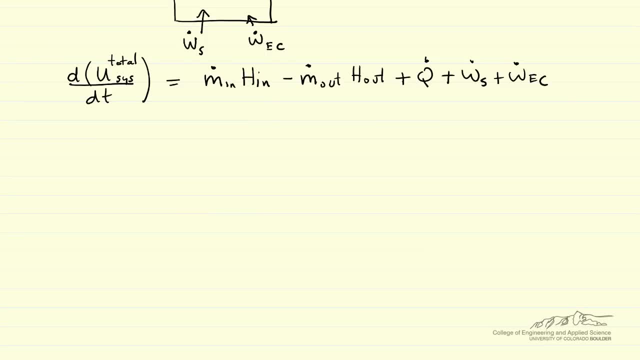 That's important, And then the other terms that we talked about: the heat, the shaft work, and the expansion, the pressure work. So what we want to do to better understand this, let's apply it to a few situations. This is a general equation, but it reduces when we have restrictions on our system. 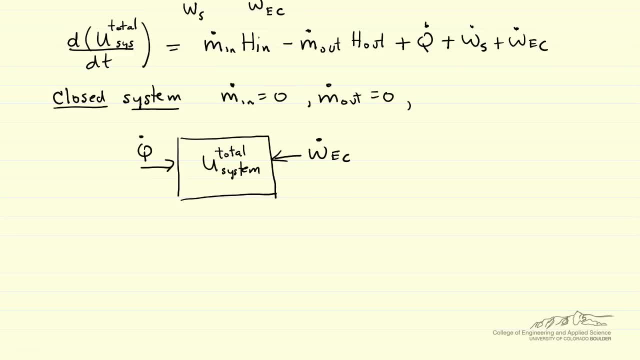 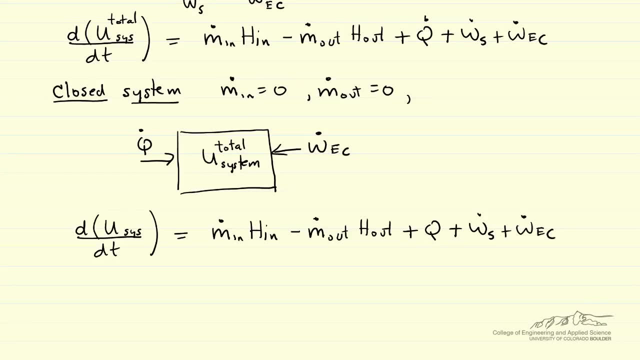 So let's look at some examples. So this first example is for a closed system. So I've written down the general equation and what we're going to do is: this is zero, this is zero, no flow in. and then I'm going to look at the special case where this is. 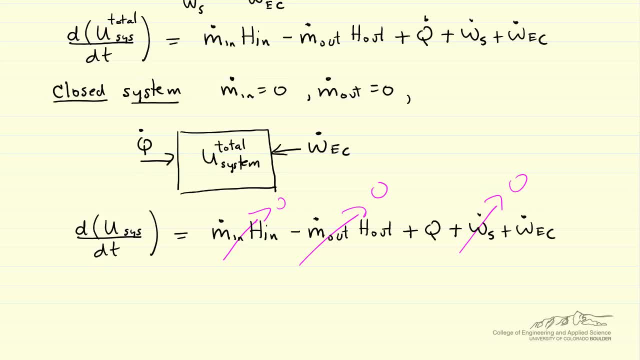 all zero. It does not have to be. we could have a propeller, excuse me, we could have an impeller that's mixing something up and adding energy, but let's look at this case And so then the equation reduces. So first let's make sure this is the total. this is not per kilogram. 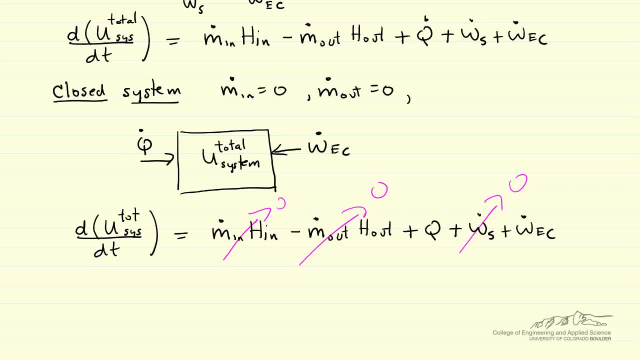 So then, let me write down. Let me write down the reduced equation. If I were to integrate this over some time period, then the left side would be delta U, total, And that would be the total amount of Q and the total amount of work that we added to. 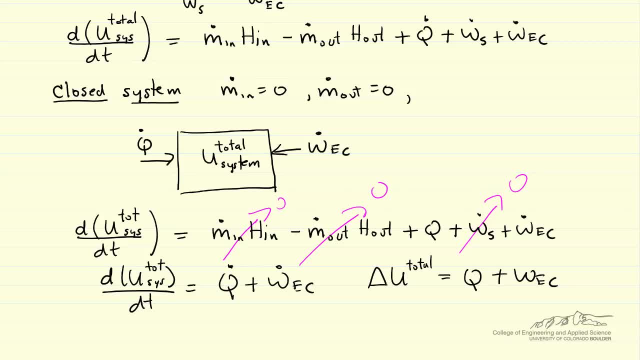 the system And we often look at this on a per kilogram basis. So now I'm going to add 20.. I'm using U to represent the kilojoules per kilogram and let me just use Q with a marked indicate. we're talking about now per kilogram, so all these are per kilogram and put this: 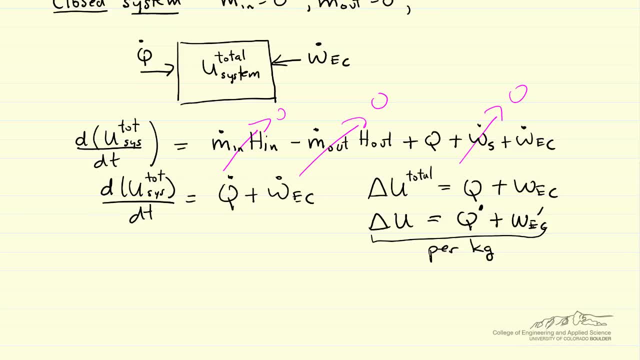 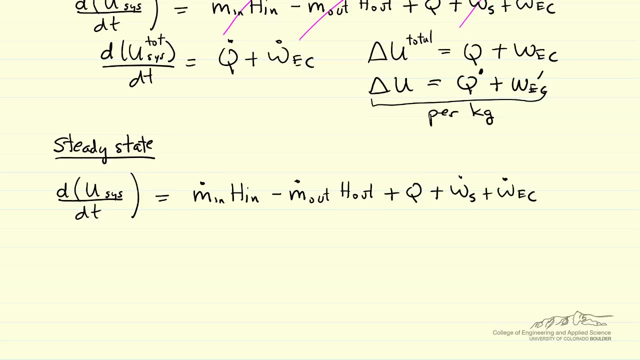 here because this is often how we look at it in systems when we do analysis. So that's one case. let's look at another case if we have a steady state system, which is certainly very common in chemical engineering processes. So we're looking at steady state system and I've written down again, copied, the general